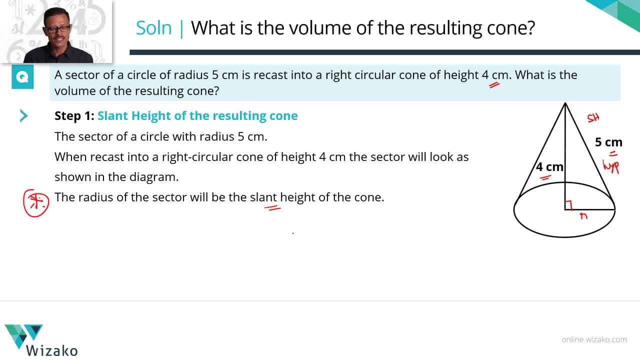 One of the perpendicular sides is the height, The other perpendicular side is the radius. So step 1, let's compute the radius of this right circular cone. So I'm going to compute the radius. Apply Pythagoras theorem. Pythagoras theorem is square root of the hypotenuse square. 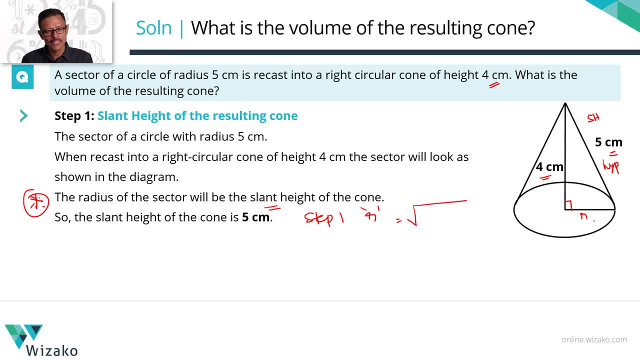 minus one of the perpendicular sides should give us the value of the other perpendicular side. R is one of the perpendicular sides. Hypotenuse in this case is equal to 4 cm. So in this case is the slant height, which is equal to 5.. So 5 square minus the measure. 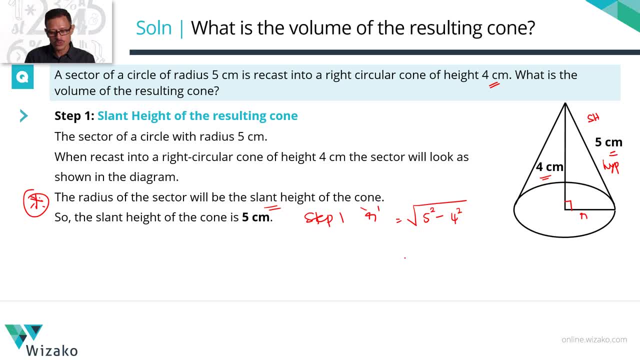 of one of the other perpendicular sides, which is the height here, which is equal to 4 square. 5 square is 25.. 4 square is 16.. 5 square minus 4 square is 25 minus 16, which is equal to. 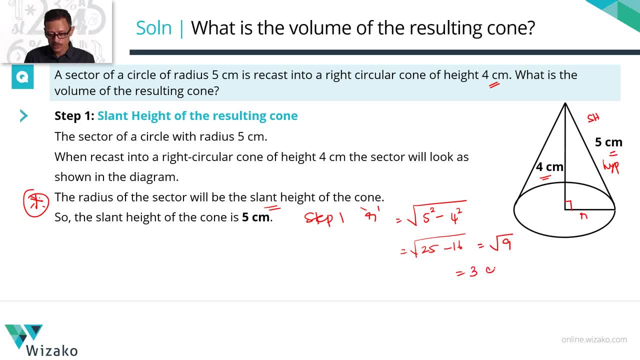 square root of 9.. Radius is square root of 9.. Radius is equal to 3 cm. So compute the radius. This is step 1 done. Step 2 is to plug in the value of the radius and height into the formula to compute the volume of the cone. Quickly summarize this bit before. 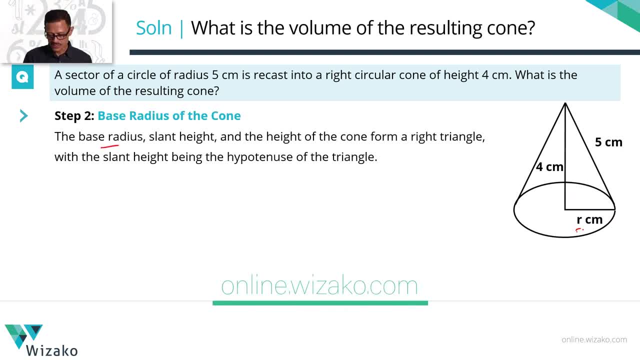 we go into computing the volume, The base radius, which is this Slant height, and the height of the cone, will form a right angled triangle. Right angled here, Slant height is the hypotenuse and these two are the perpendicular sides. Applying Pythagoras theorem, Computing the radius of the cone: 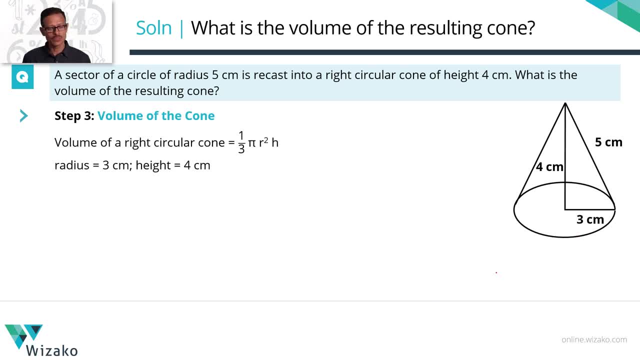 to be equal to 3 cm, Step 2.. Let's find out the volume of the cone. Volume of the cone is equal to 1 by 3 pi r squared h, which is 1 by 3.. If you took a look at the answer options, 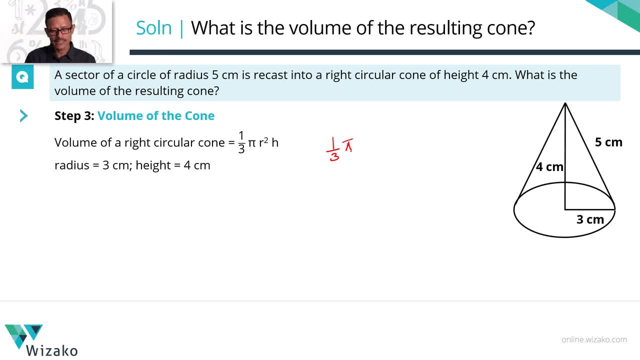 all of the answer options are given to us in terms of pi, So let's keep pi in terms of pi. If the answer had been in numbers without a pi in it, then it would have required a conversion 1 by 3 pi into the radius, which is 3, 3 square into the height, which is equal. 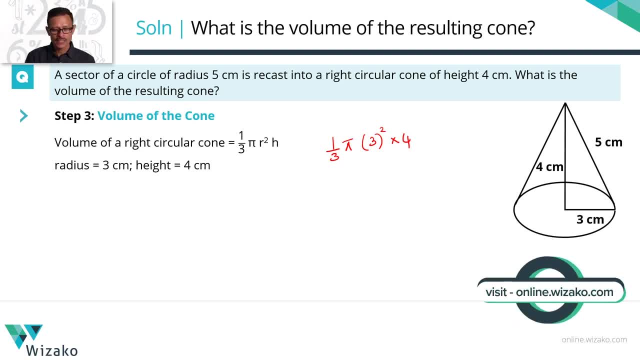 to 4.. 1 by 3 times pi times 3, square times 4.. The 3 in the denominator will get cancelled with one of the 3's in the numerator, So the answer is going to be 3 times 4 times. 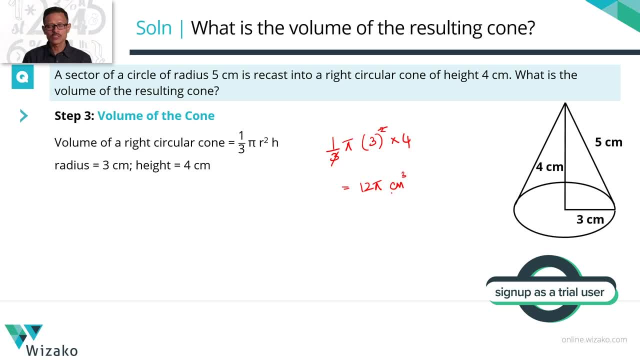 pi, which is equal to 12 pi cm cube. So volume of the cone is 12 pi cm cube. Quickly summarize it in a printed form. Plugging in the value of radius and height, we get the volume to be this Answer: option A is the correct answer. Quickly recap the key takeaway from this question.